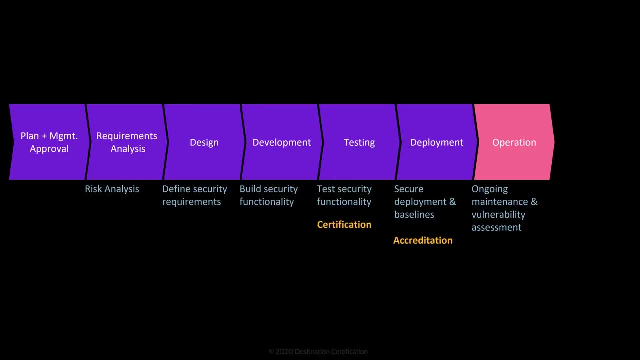 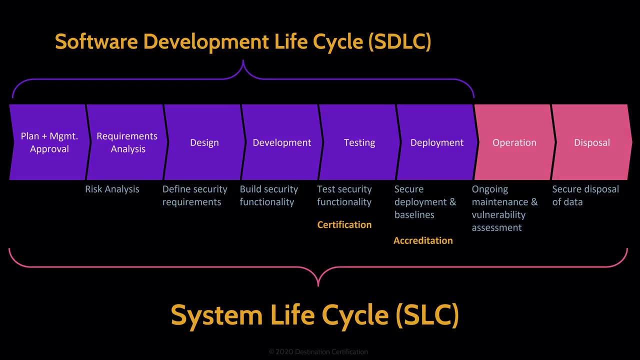 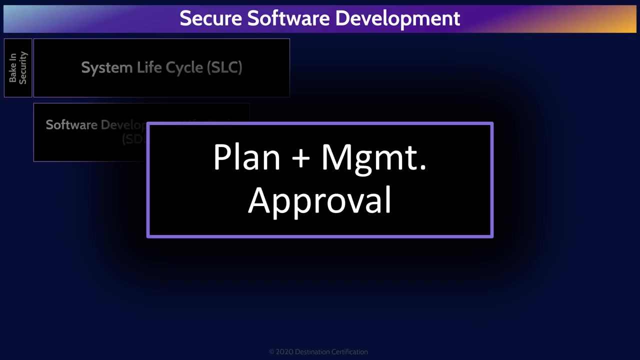 development, testing, operations, maintenance and eventual disposal of the system. The software development lifecycle SDLC, as the name implies, focuses on the development phases Starting with defining a plan for a project. What goals and objectives will the project help the organization achieve? What are the high level cost estimates? 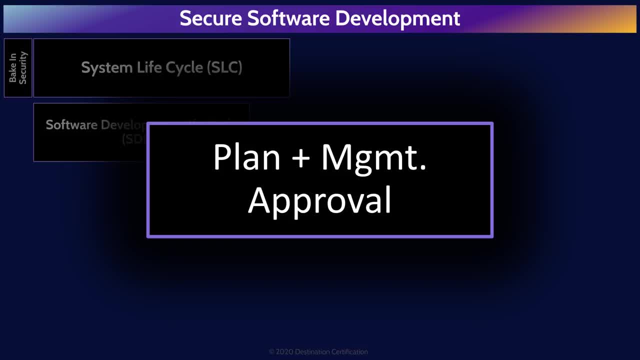 And obtaining management approval to proceed with the requirements analysis. The requirements analysis phase is where business requirements, user needs, the type of data to be collected, stored, processed, the business uses of the system and so forth Are gathered and validated to create a detailed set of requirements. 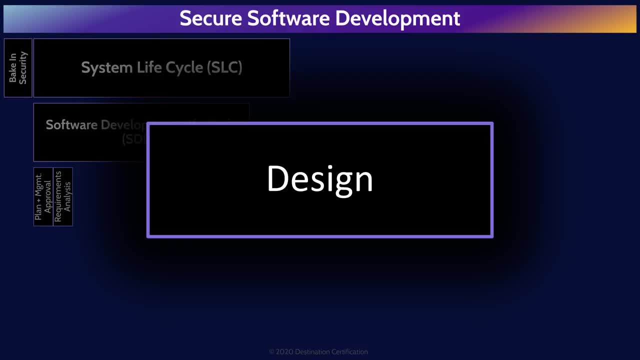 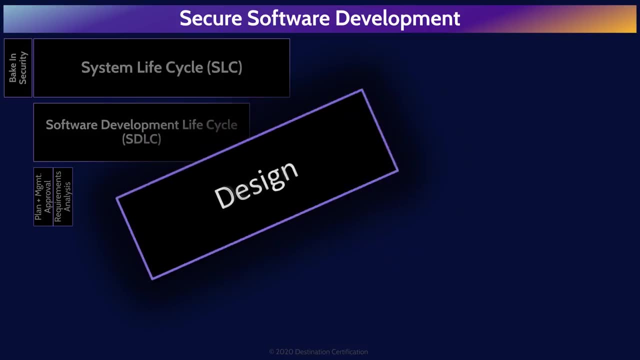 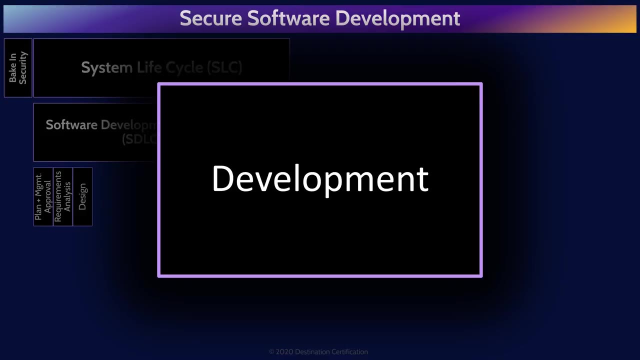 The design phase is where requirements are transformed into detailed system design documents, including the architecture, security controls, screen layouts and so forth. the development phase is where the coding begins writing the code to create the system. there are many methodologies that have been developed over the years to 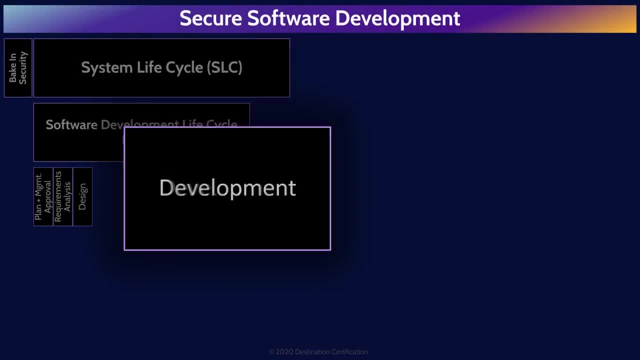 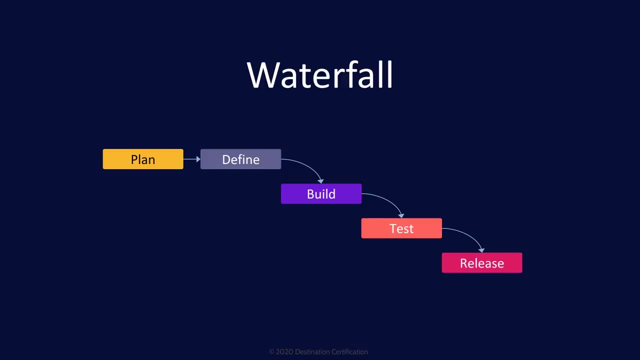 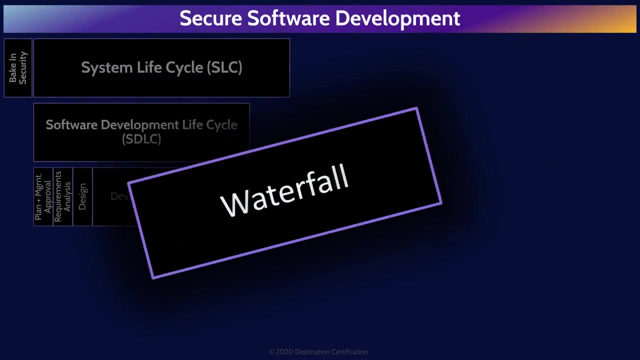 guide the development process and I'll cover just a few key ones. waterfall begins with a plan, then defining requirements, building, testing and finally releasing. the defining characteristic of waterfall is that each of these phases are conducted one after another. you cannot go backwards. water can only flow downhill. so if you discover, as part of a two-year waterfall, 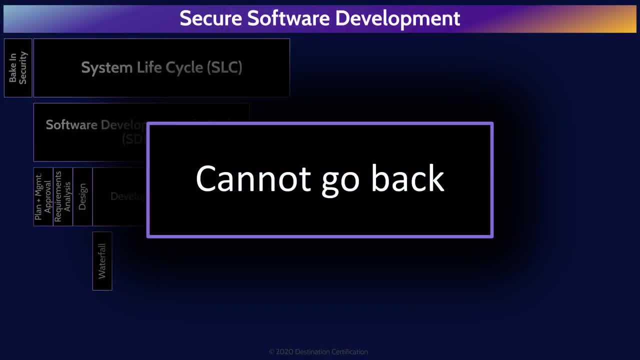 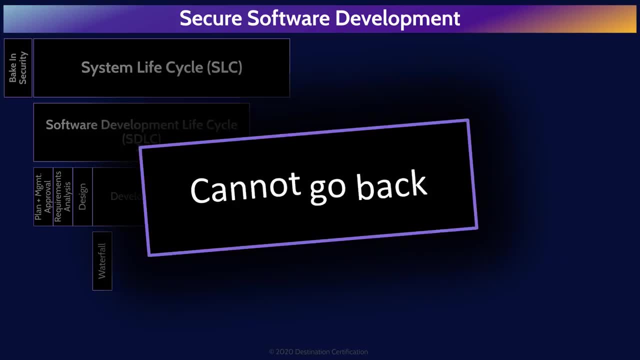 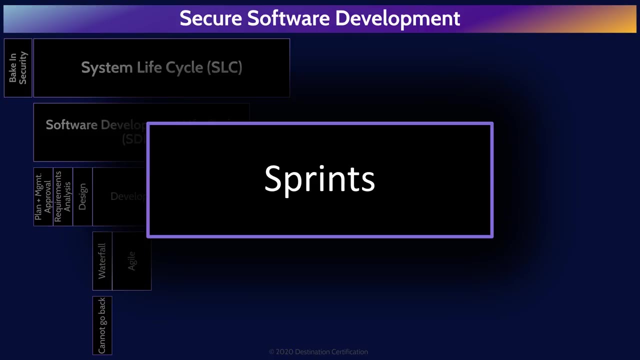 project that you missed a requirement. you can't go back and redefine the requirements. you must proceed through build, test and release and then include the missed requirements as part of the next waterfall cycle. agile was created to address this problem. agile follows exactly the same phases as waterfall, but 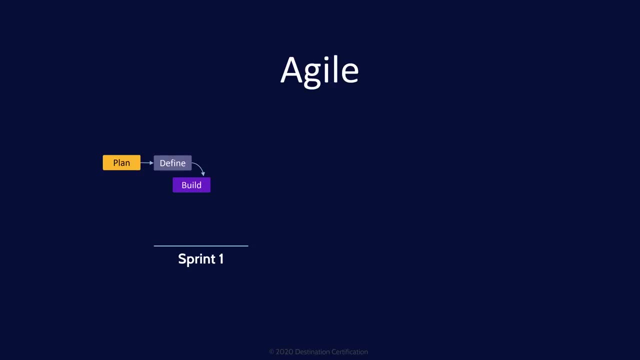 does them in typically two week sprints. rapidly iterating through plan, define, build, test and release. waterfall is better suited for projects where no changes are planned and agile is better for projects where many changes are expected, where organizations want to rapidly iterate ideas and fail fast through rapid sprints. agile includes the 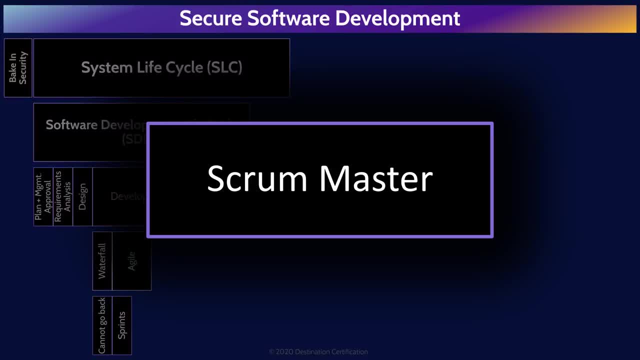 role of a scrum master. this person is a facilitator, and I'm intentionally emphasising the word facilitator. a scrum has no real authority over the team. They are not project managers, but rather they're to act as a coach to the team and facilitate communications with the organization to maximize the productivity. 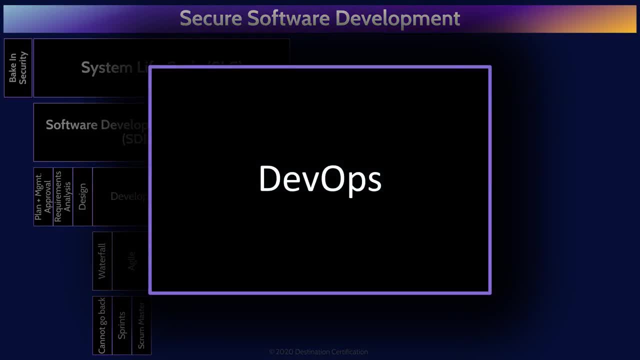 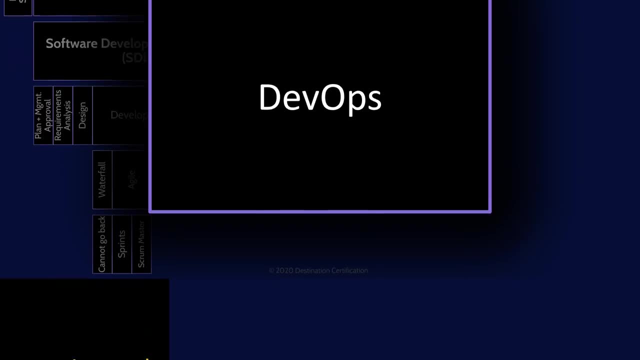 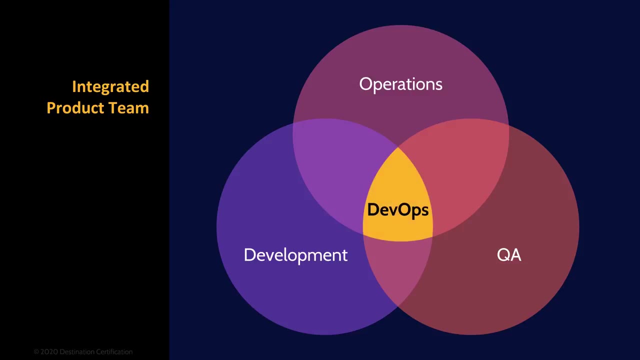 of the team And, of course, the latest and debatably greatest software development methodology is DevOps. This is what all the cool kids are doing. DevOps, as the name implies, combines development- the dev part, quality assessment and operations- the ops part- to significantly shortened development. 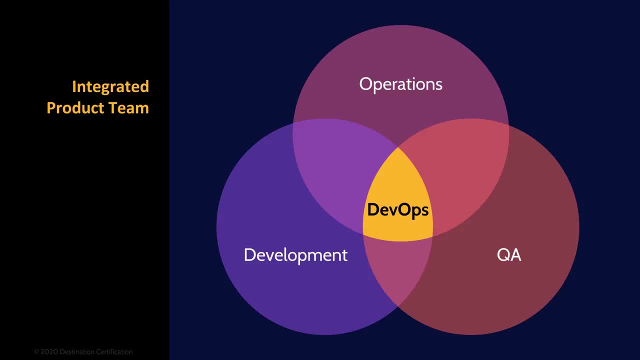 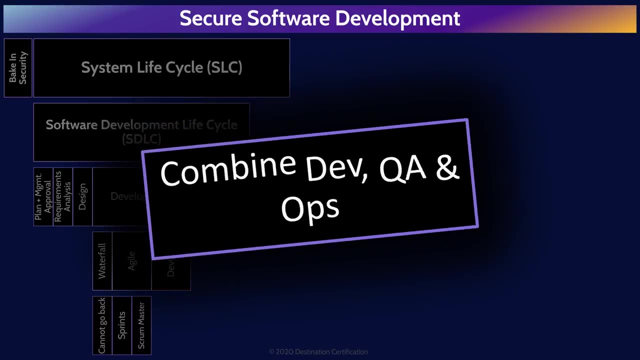 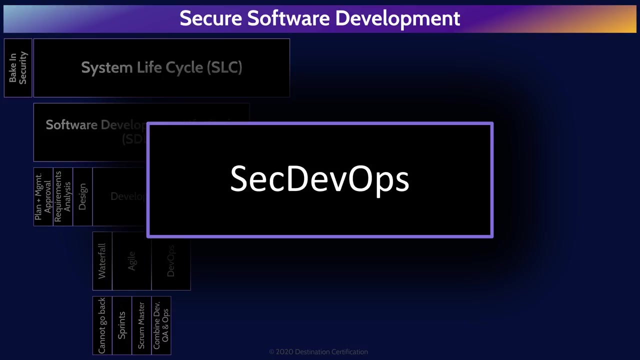 lifecycle, possibly to the point of releasing new code daily, or even more so. DevOps includes automated practices such as continuous integration and continuous delivery. DevOps can seem contradictory to having security in the development process, as sacred security practices like segregation of duties between development and operations are intentionally removed And many 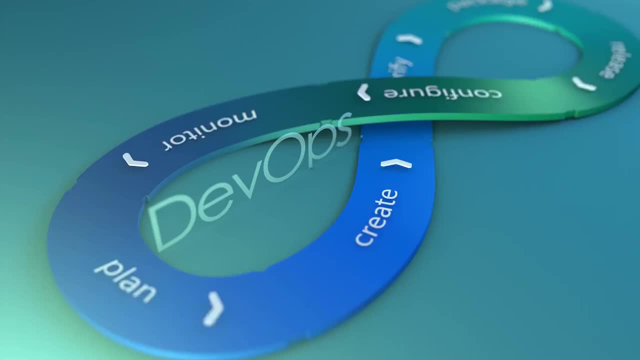 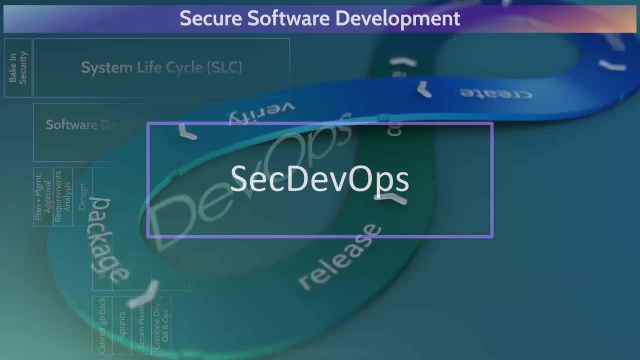 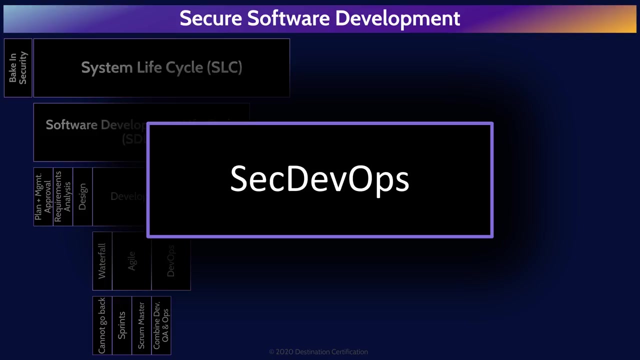 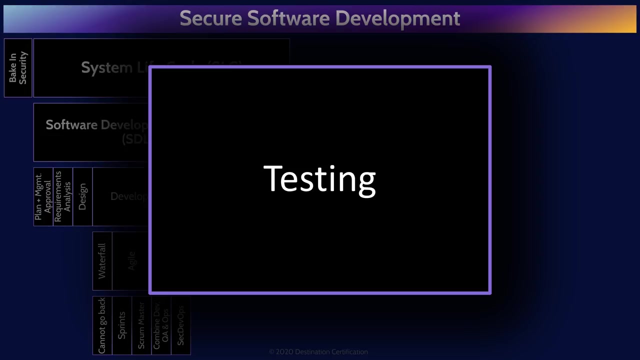 other traditional security techniques are too slow to fit into the rapid iterations of DevOps. Therefore, integrating security into DevOps requires strong engagement between developers and security using secure software development frameworks, automating much of the security testing and only using traditional security testing techniques, such as penetration testing, sparingly. It is very important to test throughout. 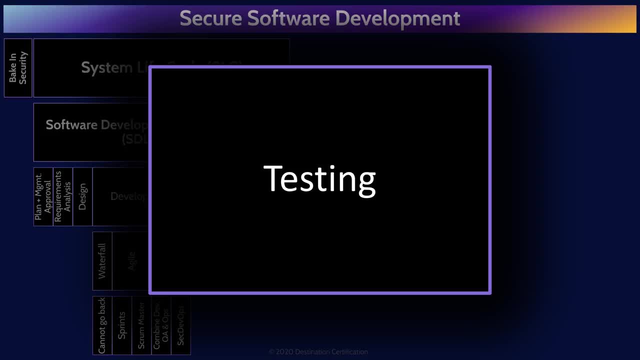 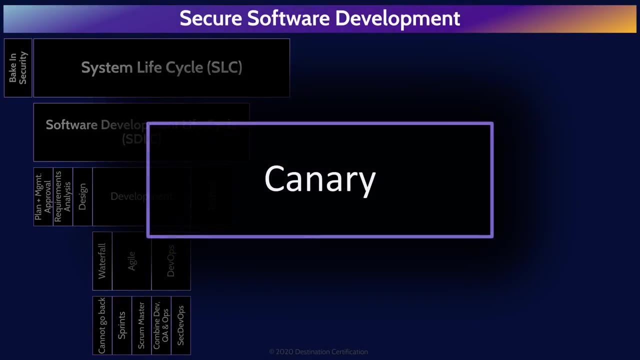 the system lifecycle, from validating business requirements, reviewing designs, testing units, interfaces, integration and the whole system during development and operations. I cover these various testing techniques in detail in the first video for Domain 6, which I've linked to. One particular software development testing technique that I want to highlight is canary. 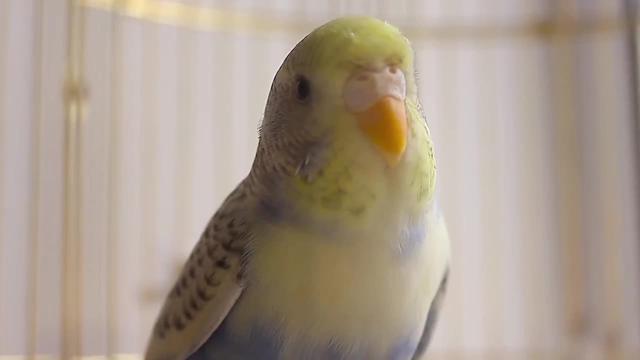 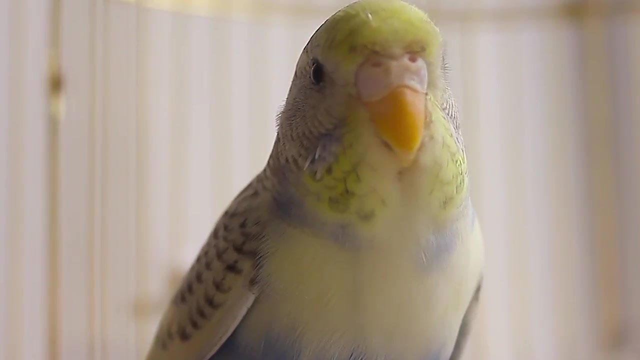 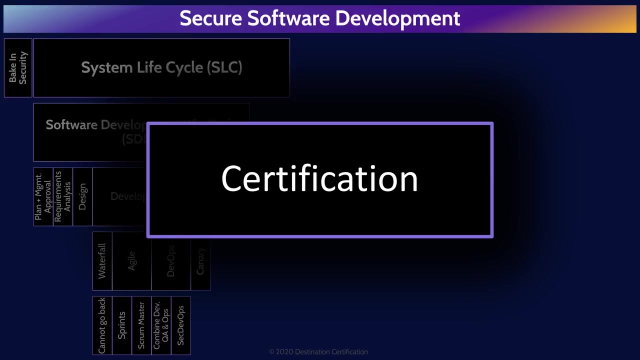 deployments. The idea is to gradually release new features to a subset of users as an early warning system to see if anything breaks before releasing to a wider audience, like the canary in a coal mine. An important topic that I'll cover in Domain 3 are eval trivial criteria, Basically independent, objective evaluation and measurement of vendor. 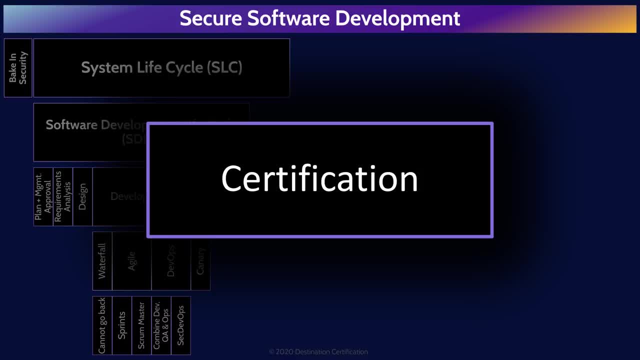 products from a security perspective. These evaluations involve two major steps. The first is certification, which is an independent, comprehensive technical analysis of a solution or product. Certification fits here under testing within SDLC. The second part of eval criteria, accreditation, fits under deployment. Deployment is the final. 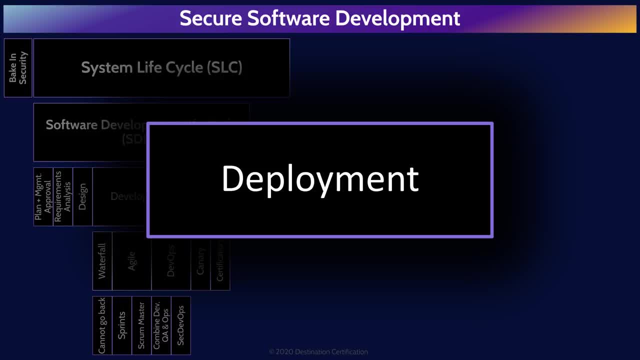 stage of the software development lifecycle, and deployment is where a system is moved into production. Accreditation is the official management sign-off of certification for a set period of time. In other words, accreditation is where management says yes, we sign off on this. 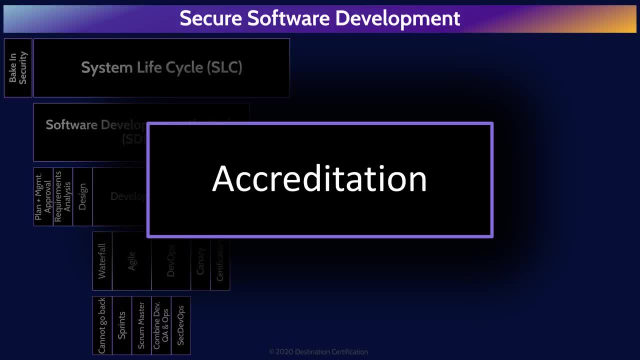 particular product being used in production for this period of time. So this accreditation step fits here. under deployment Operations is where the system is being actively used for business purposes. It is in operation. The disposal phase is extremely important and often overlooked. When a system is retired and replaced, there needs to be controls in place to ensure data. 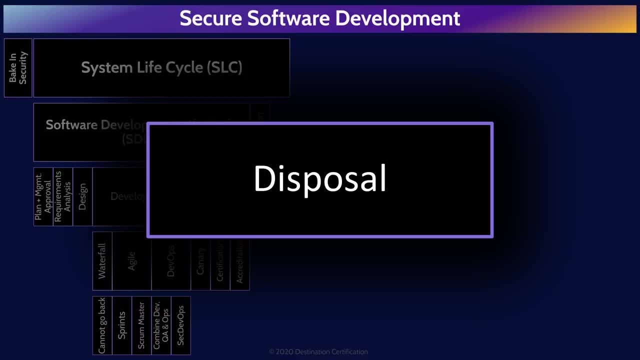 logic, processes etc. are migrated to the new system with integrity. Data in the old system is retained as necessary, and if the old system and data are to be deleted, the data may need to be defensively destroyed and not just left on a hard drive that is then sold on eBay. 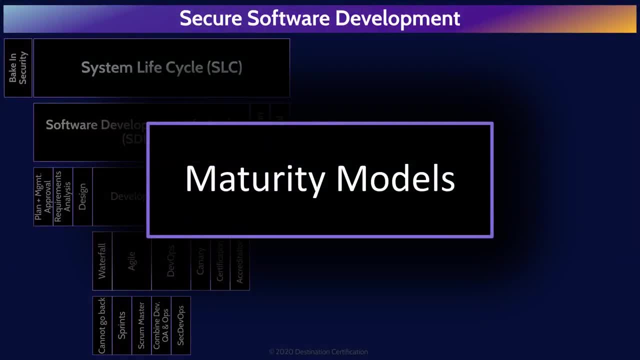 Hard drive: Hooray for privacy breaches. Maturity models can be a useful tool in software development and operations. Maturity models enable the repeatable evaluation and benchmarking of processes using well-defined levels, starting at the bottom, with level 1, which is called initial or 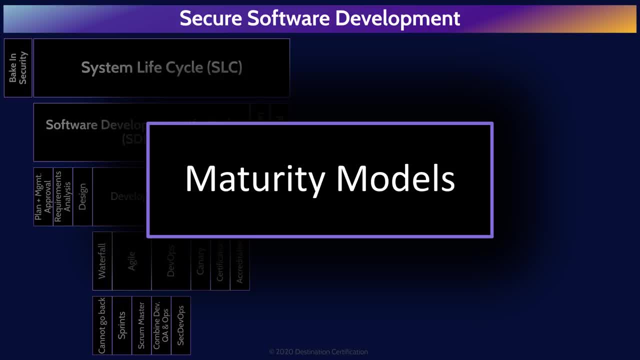 ad hoc and moving up through 2, repeatable, 3, defined, 4, managed and 5, optimized. Level 1 ad hoc basically means you have no processes and it is barely controlled chaos. And the other end of the spectrum is level 5 optimized, which is an uneconomical and unobtainable 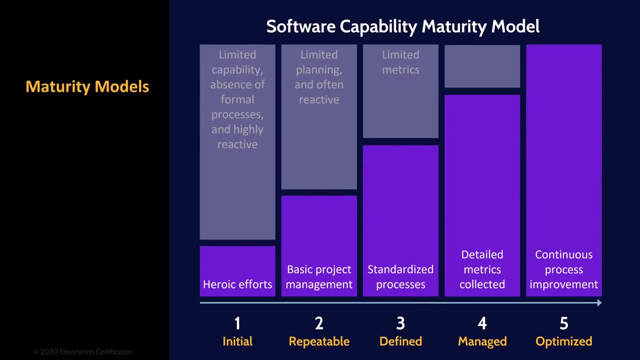 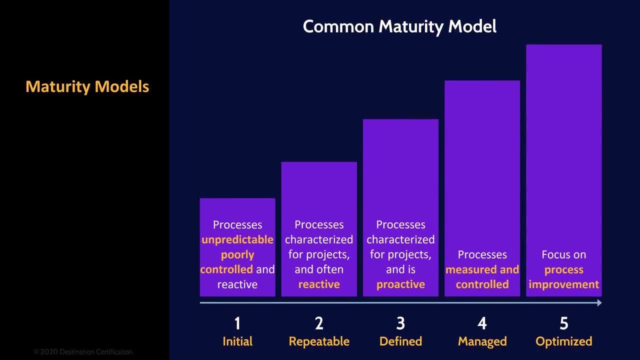 goal for most organizations. Here is a maturity model specific to software development and here is a more generalized common maturity model for various types of processes across an organization. I would pay particular attention to this common maturity model as it is very commonly used in organization and it is not uncommon to see questions on the exam about this. 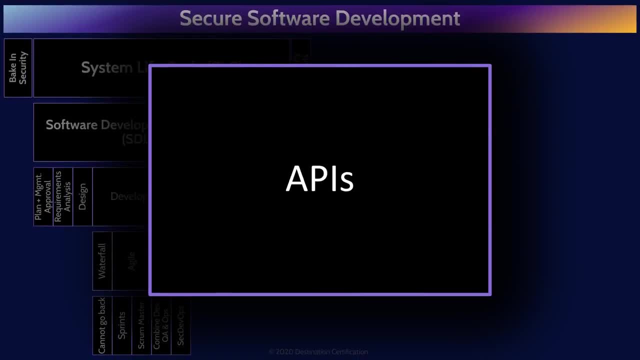 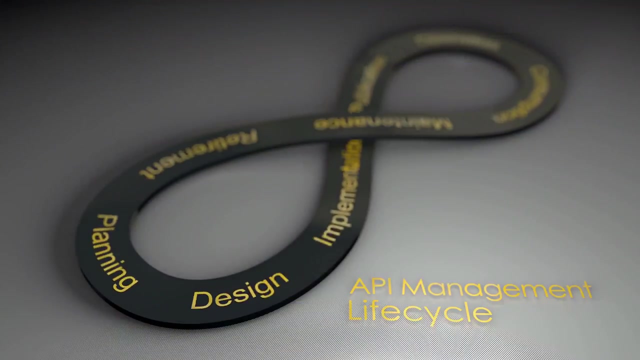 model and its levels. Now let's talk about the process of maturity. Let's talk about application programming interfaces, APIs, which are the system of tools and resources which allow two applications, for example a client and a server, to talk to each other across a network. APIs are used pervasively in software development as they 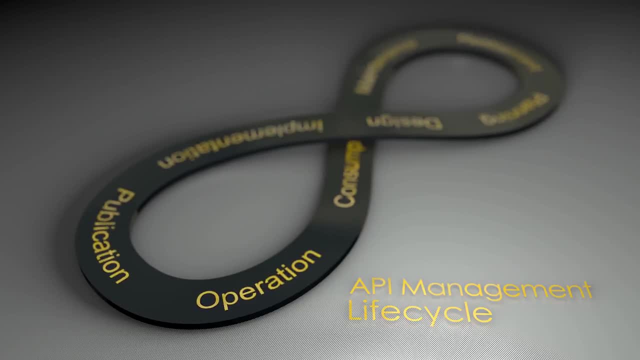 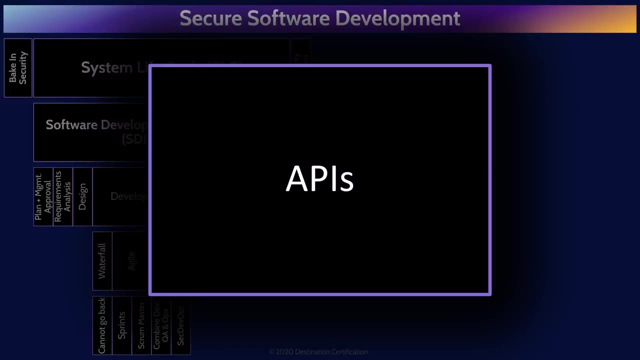 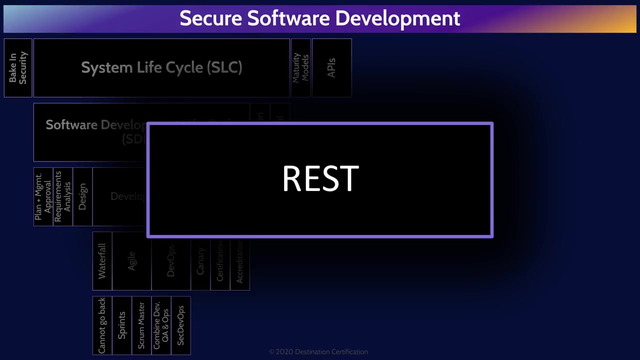 enable developers to make repetitive yet complex processes highly reusable with just a little bit of code. There are two major protocols used for creating APIs: REST and SOAP. Representational state transfer: REST is the most commonly used and is lightweight and fast. Simple object access protocol. SOAP is 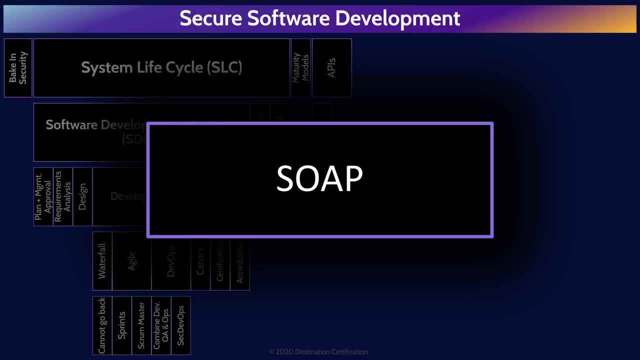 far more complex and heavyweight, but accordingly provides a lot more capabilities. Code obfuscation is the deliberate act of creating code that is difficult for humans to understand. Why on earth would we want to do this? To make code more difficult to reverse, engineer and. 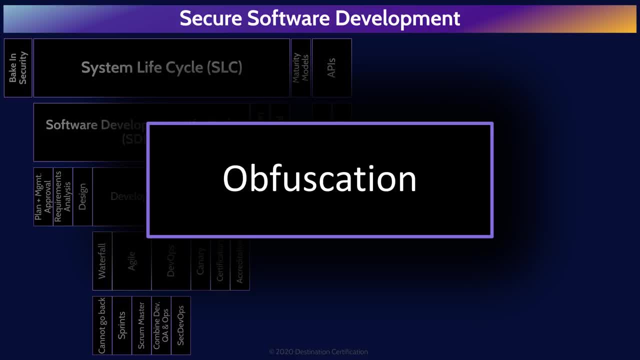 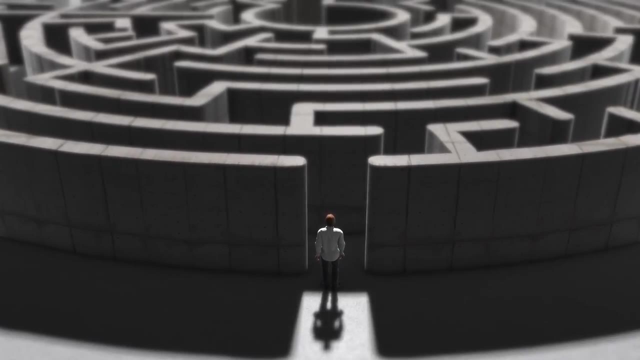 conceal the purpose of the code. Code obfuscation is used when we don't want unauthorized people to understand how our code works and what it does. There are three major methods for obfuscating code. Lexical obfuscation modifies the look of the code. changing comments, removing, debugging. 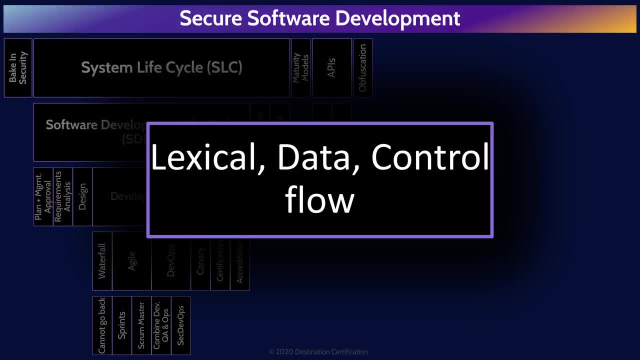 information and changing the format of the code. Lexical is the easiest to do but weakest form of obfuscation. Data obfuscation modifies the data structure, use of variables, etc. And control flow modifies the flow of control through the code, reordering statements, methods, loops. 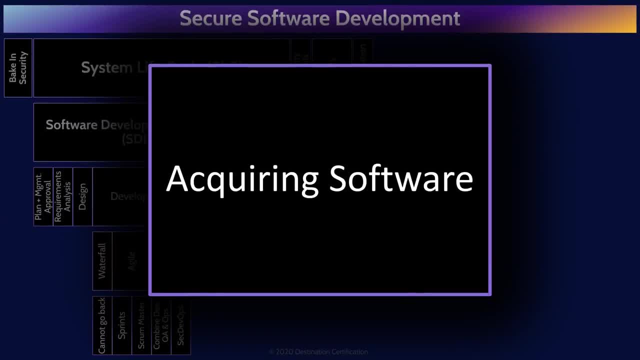 and creating irrelevant conditional statements. If an organization is acquiring code by contracting an organization to write custom code or buying some off-the-shelf product, then the organization needs to conduct some software assurance activities to ensure the code is free from vulnerabilities and functions as intended. An important part of this process is assessing 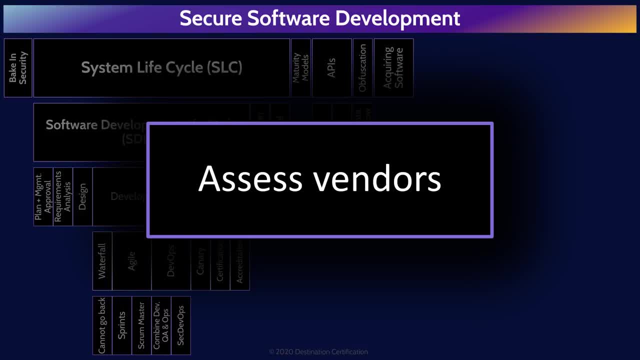 the vendor that is providing the code, to ensure they use secure software development techniques sufficiently, test their code and so forth. Contracts and SLAs are another important tool that an organization can use to define the controls that a vendor must have in place and measure the effectiveness of these controls through metrics. 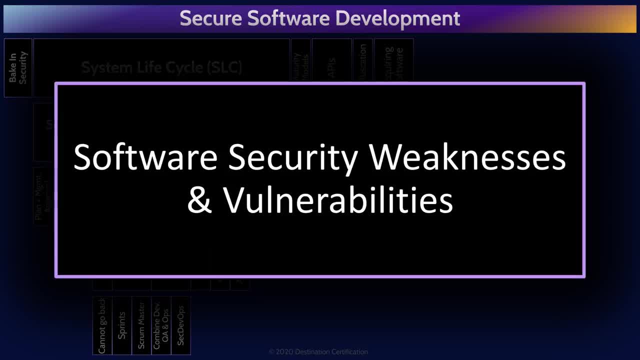 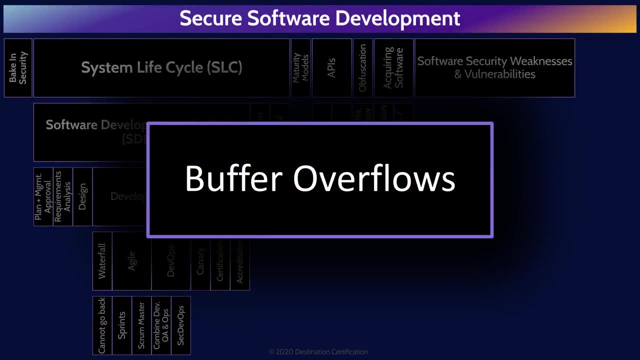 and reports. Now let's talk about some common software security weaknesses and vulnerabilities that we need to ensure we put controls in place to avoid while developing software, and tests we can conduct to detect during the development and operational phases. Buffer overflows is a condition where a program, while writing data to a software, is not able to detect the controls that a vendor. 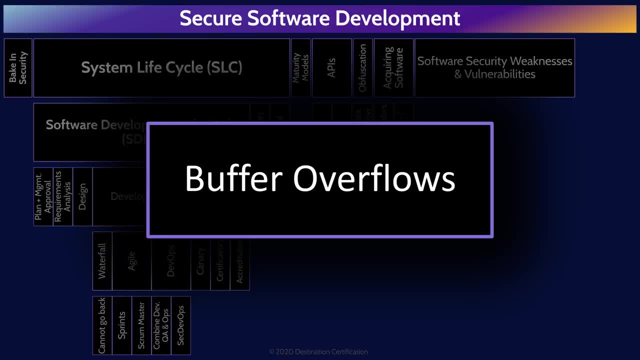 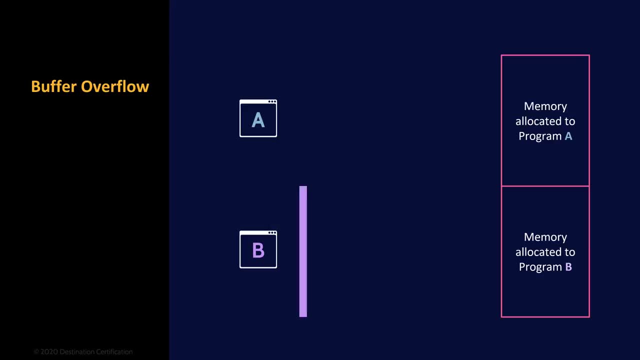 actually uses to fix. You might notice that a buffer-to-memory operation overruns its boundary and overwrites data into adjacent memory locations. Here's a diagram that shows what that looks like. Put more simply, a program attempts to write a chunk of data to a buffer and the 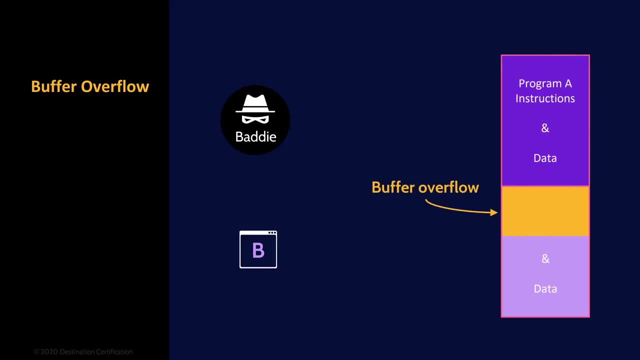 chunk of data is larger than the buffer. Risk occurs when the overwritten data is read and executed by another program. To protect against buffer overflows, code should always be written to perform parameter or bounds checking. To never allow a buffer to bump out, you should always write your. 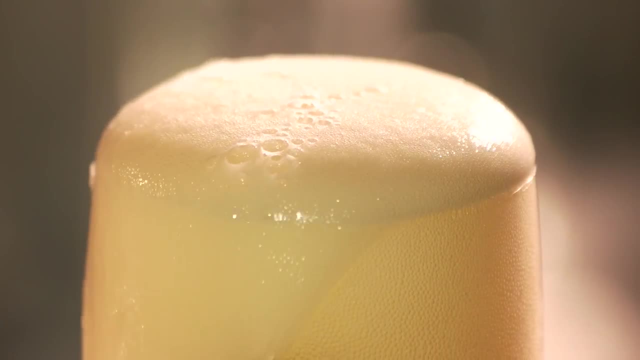 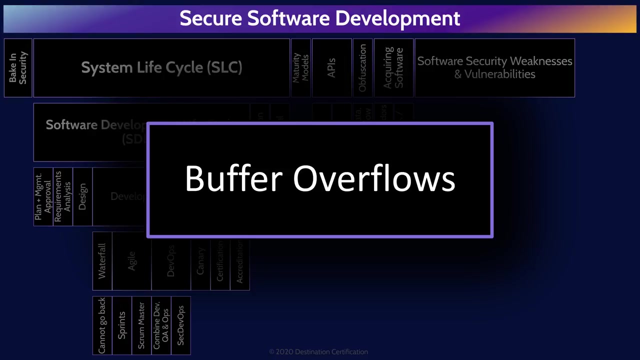 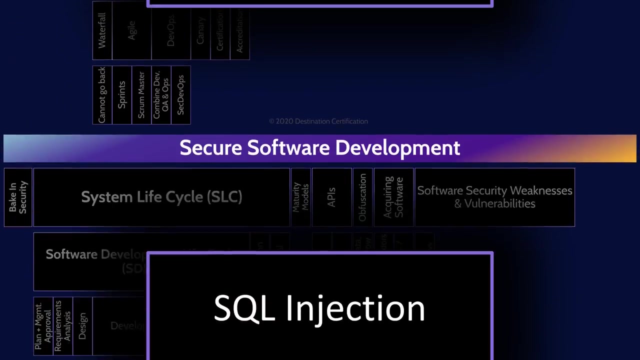 allow a chunk of data to be written to a buffer that is larger than the buffer. Another technique that can be used is Address Space Layout Randomization, which guards against buffer overflow attacks by randomizing the location where system executables are loaded into memory. 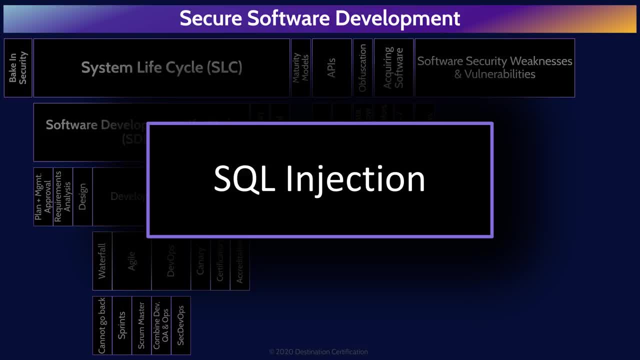 SQL injection is where malicious Structured Query Language code is inserted into a form field on a website, sent to the web application, and then the web application passes the malicious SQL code onto the database, essentially allowing the T attacker to directly control a database that they should have no ability to control. 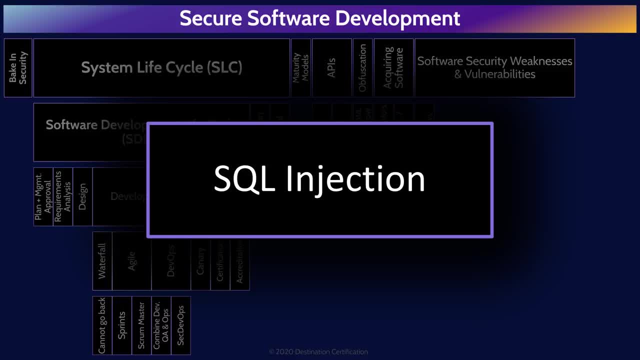 I'll be creating more detailed videos on SQL injection and the next few topics- cross-site scripting, cross-site request, forgeries, covert channels and backdoors- as part of domain 3.. I'll link to those videos when they're done. The major way to prevent SQL injection is to perform input validation. 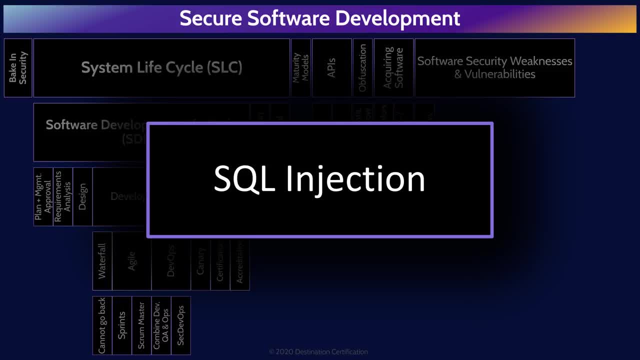 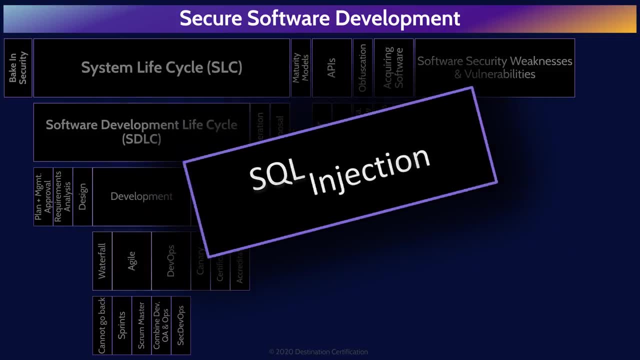 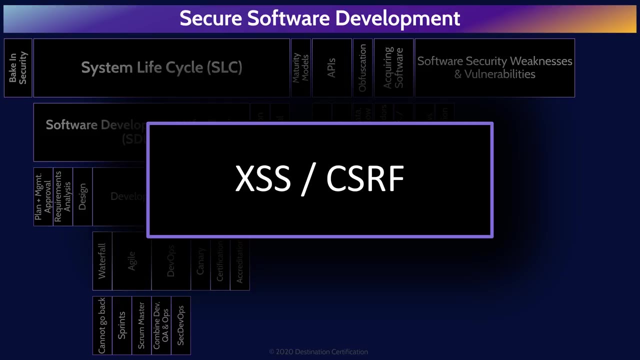 The web application should never allow SQL code from a user to be passed directly to the database. Input validation is also how we protect against the next topic: cross-site scripting. Cross-site scripting attacks allow an attacker to inject client-side scripts into web pages viewed by other users. 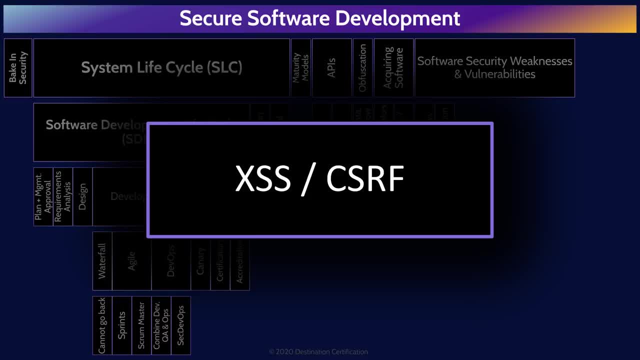 This causes the malicious code from the attacker to be executed by the victim's browser. There are two major flavors of cross-site scripting that you need to know about: stored and reflected. Stored is persistent and reflected is more common. All flavors of cross-site scripting target the victim. 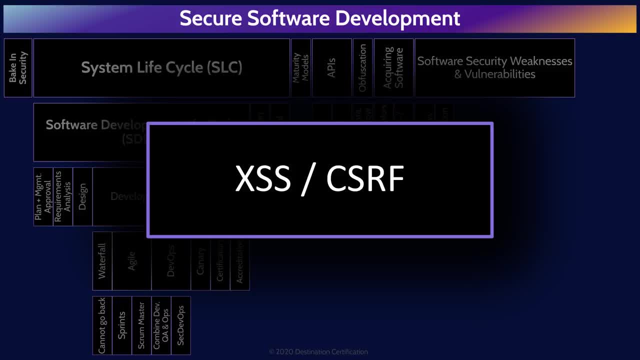 Cross-site request forgery attacks, on the other hand, target a web application. This is accomplished by tricking a valid and authenticated user into sending some commands to a web application that trusts the user. The web application executes these commands from an attacker that it shouldn't be executing. 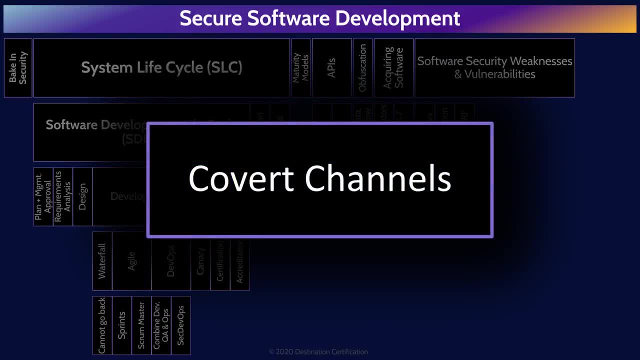 Covert channels are unintentional communication paths that have the opportunity to disclose confidential information. There are two major types of covert channels. The first type of covert channels is the one that is used by the attacker. It is the most common type of covert 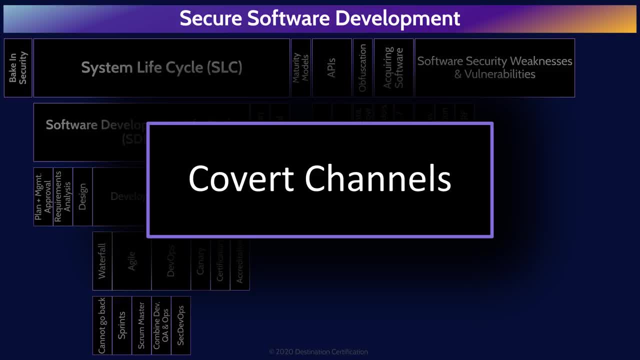 The second type of covert channels is the one that is used by the attacker. The third type of covert channel is the one that is used by the attacker. The fourth type of covert channel is the one that is used by the attacker. The fifth type of covert channel is the most common type of covert 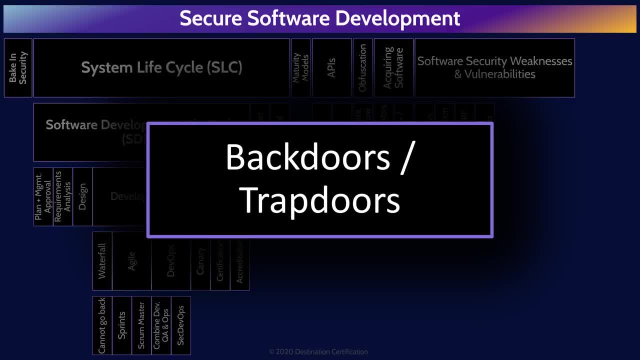 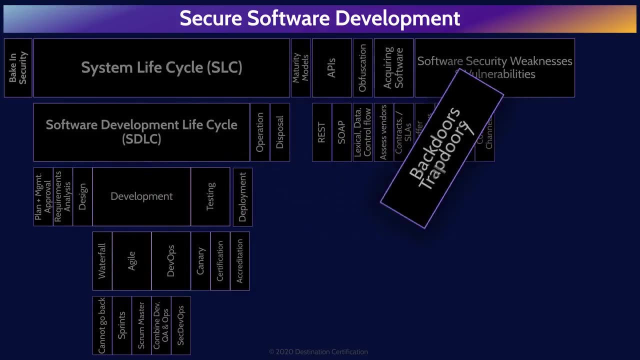 Backdoors, also known as trapdoors, are intentional, covert methods of gaining access to a system and bypassing the normal authentication and encryption controls. An attacker will install a backdoor in a system or hide one in code which allows them to gain unauthorized access to an application or system. 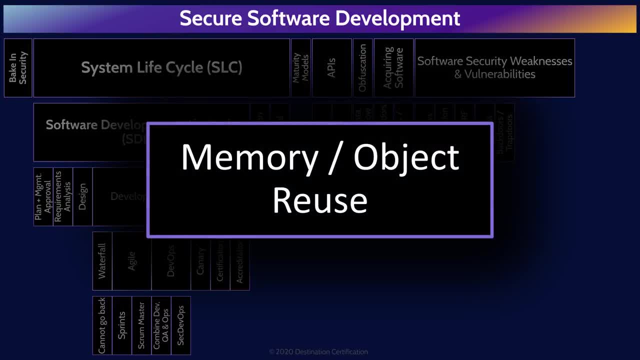 Memory reuse or object reuse is a vulnerability in the way memory is allocated to applications applications. if an application, a, has stored some data in a section of memory and then no longer needs that memory space, then the memory space can be deallocated and then reallocated to another. 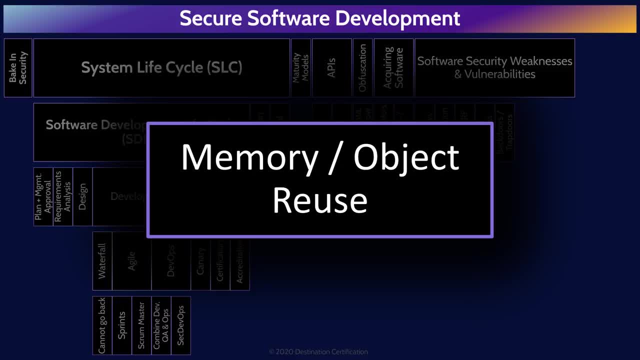 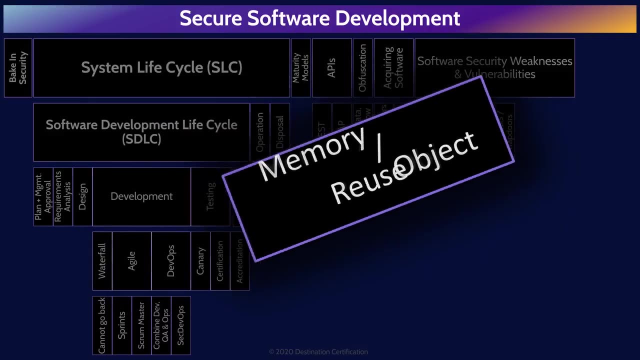 application, say application b, and the risk occurs if the data that application a stored is still in memory and is now accessible by application b. to prevent this vulnerability, the operating system should ensure memory is zeroed out before being reallocated to another application. toctow time of check, time of use, also known as race conditions, is where an application 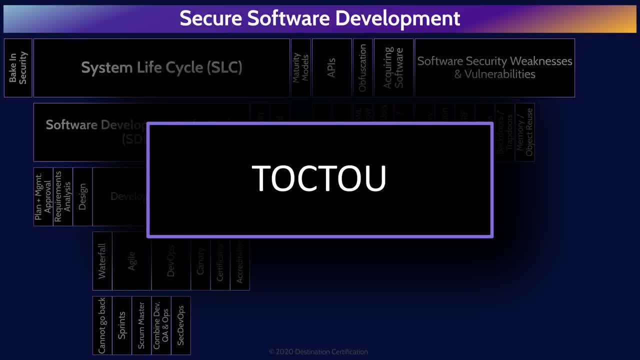 checks the state of a resource before using that resource, but the resource's state can change between the check and the use in a way that invalidates the results of the check. this can cause the application to perform invalid actions. in other words, an attacker attempts to race in. 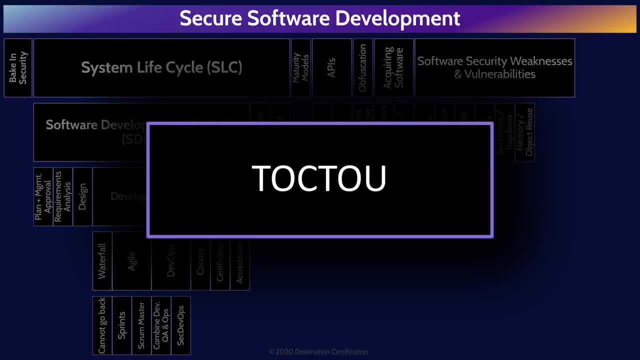 and change a resource, a file, a variable or some data in memory between when the resource is checked and used. citizen development developers are employees from business operations that are empowered to create applications through all the new tools that make programming accessible to basically anyone. the risk of citizen developers. 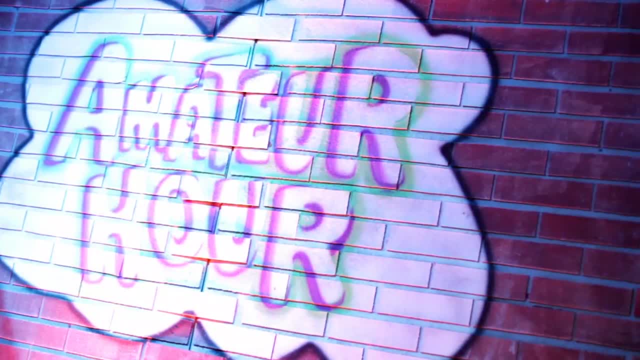 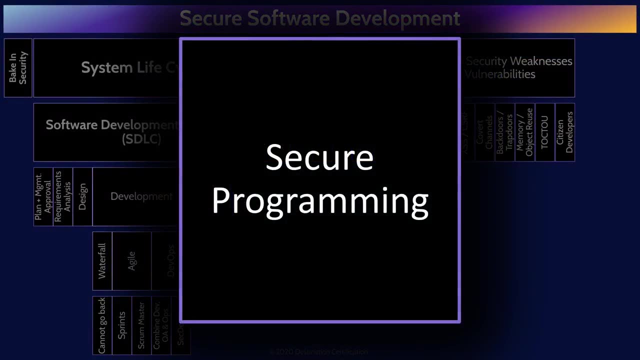 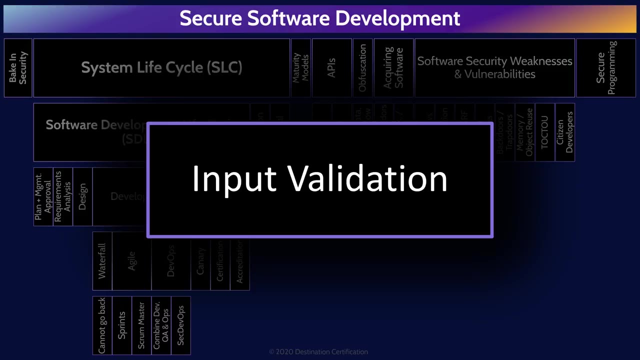